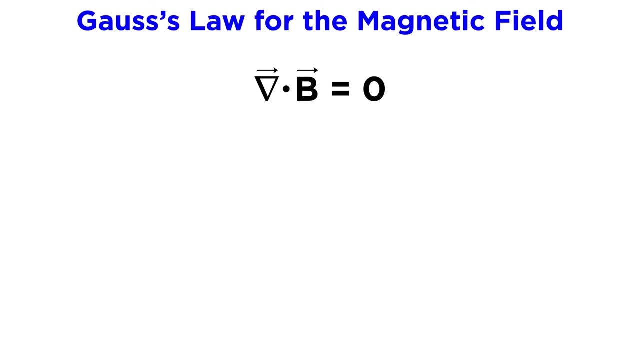 for the first of Maxwell's equations. Since the method is identical, we will just quickly summarize it here. We can integrate both sides with respect to dv, which means the right side will remain zero, and then we apply the divergence theorem, allowing us to replace: 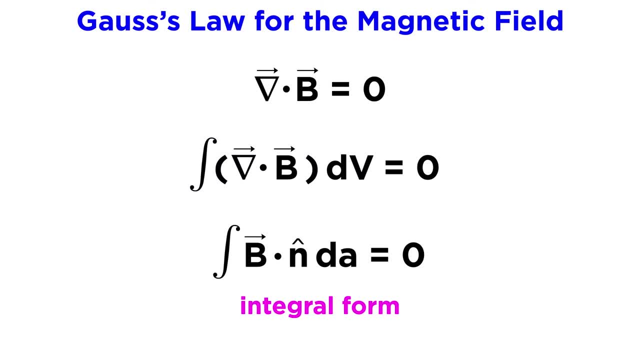 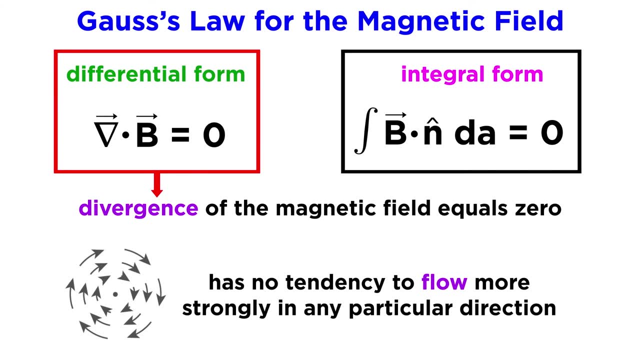 this expression with this surface integral. And there we have the integral form As a quick reminder. looking again at the differential form, we can see that the differential form is the divergence of a field, is the tendency of that field to flow more strongly away. 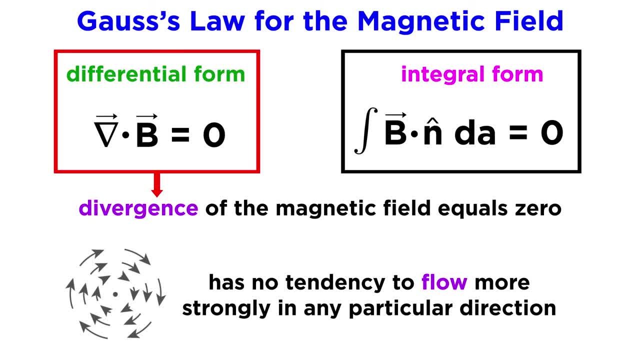 from a point than towards it. A divergence of zero means a flat field. This is an important property and it reaffirms the idea that a magnetic field does no work. There is no magnetic charge density because the magnetic field does not originate from a point source, but 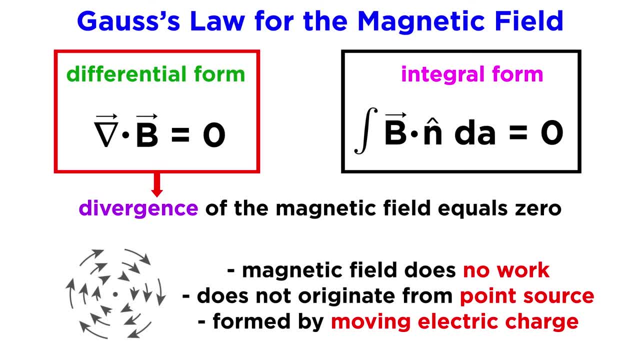 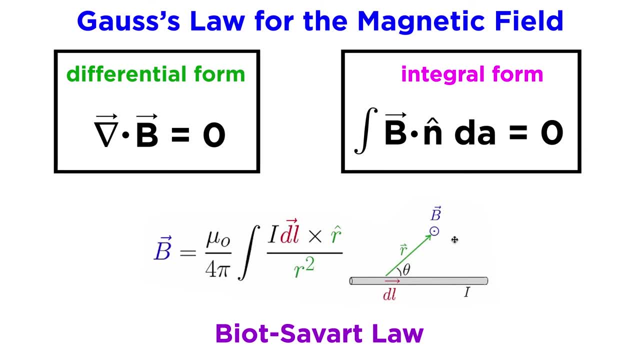 rather from a moving electric charge, which is a vector. These two equations are difficult to use directly in practice. More often, these equations are used to resolve a difficult or complex situation arising from other, more common equations, such as the Biot-Savart law, For example. if you know, the magnetic field within a part, 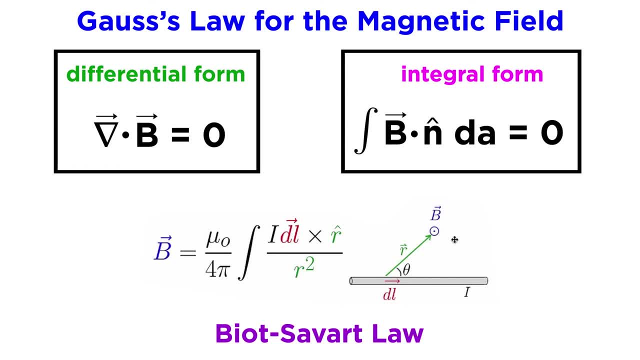 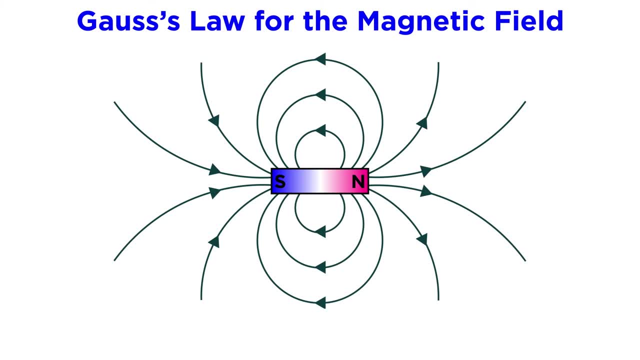 of a complex shape, Gauss's law can be used to determine the remaining field. On principle, Gauss's law for the magnetic field displays the simplest facts about the magnetic field. A great representation of the magnetic flux is the idea of magnetic field lines Unlike 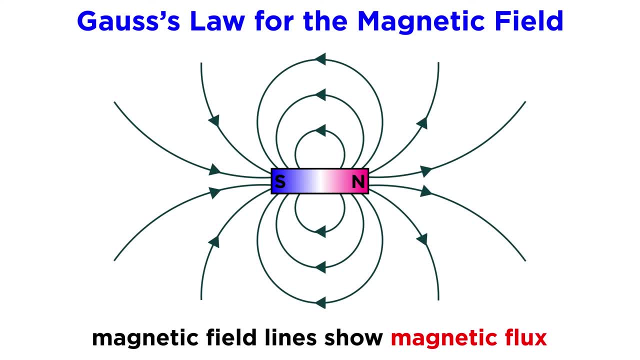 electric field lines. magnetic field lines do not terminate. They are complete loops that pass through the north and south poles of the magnetic field. No matter what closed surface one draws around these lines, there will always be an equal number of lines going out and coming in. This satisfies Gauss's law. the total flux is zero In the next two. 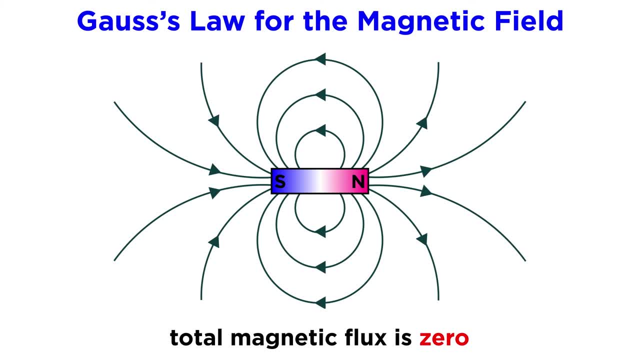 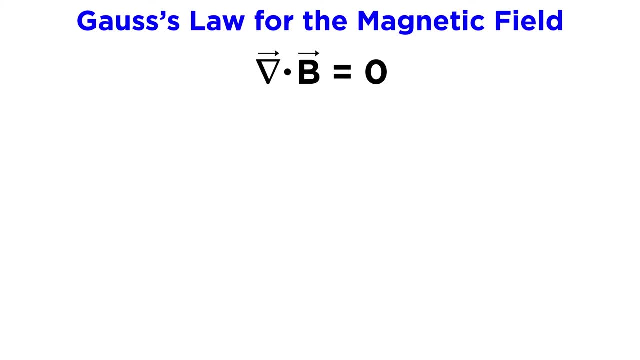 tutorials. after this video, we will discuss magnetic field lines, And after this one, the relationship between the electric field and magnetic field will be explored further. Before we get there, let's take a look at a problem using the results of the two forms of Gauss's law. Given the following expression for a vector: